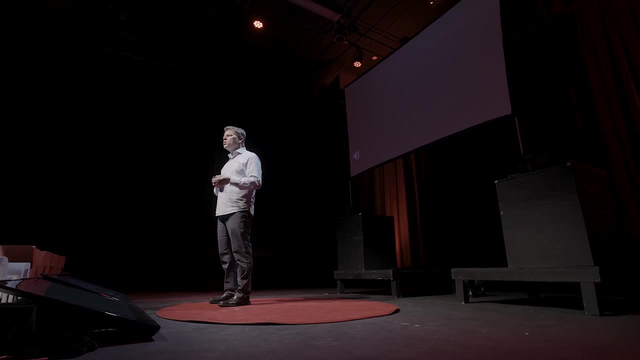 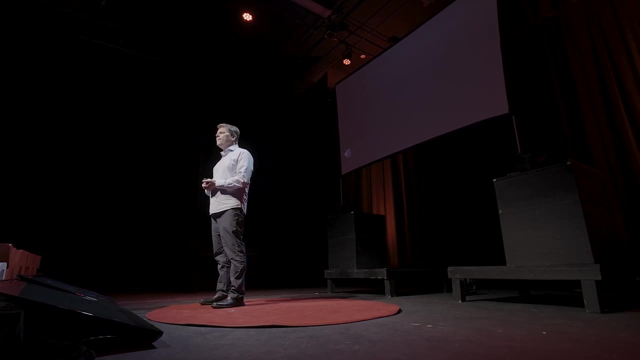 What I do know is that, for me, musical feeling is not a choice. It comes instinctively, automatically, naturally, like the act of breathing. I think what was happening growing up is I was learning about the beauty of the world through music. 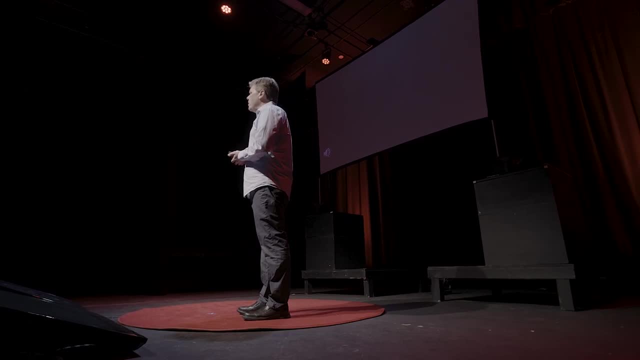 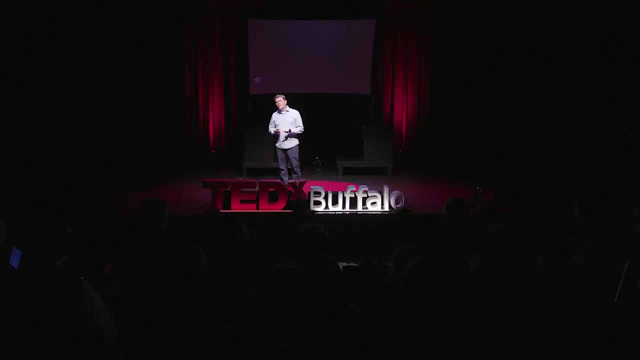 I was awakening to an innately human need for connection. I was experiencing and learning empathy. I was being educated about the human condition through music. Music is a deeply human thing. Decades of studies across disciplines have validated the place of music in our human development. 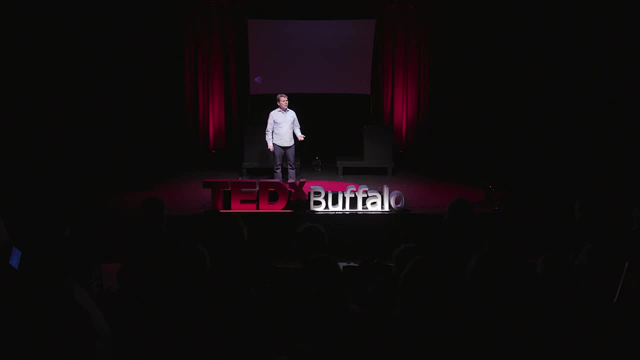 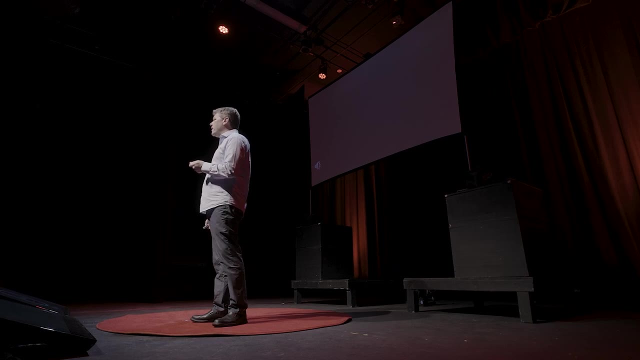 There are increasing studies which support the idea that music has biological roots and that we are indeed hardwired to enjoy and engage with music, just as we are hardwired for language. Research on many fronts supports this conclusion. There are no societies, either today or in the past, that did not have some sort of cultural practice which could be described as music. 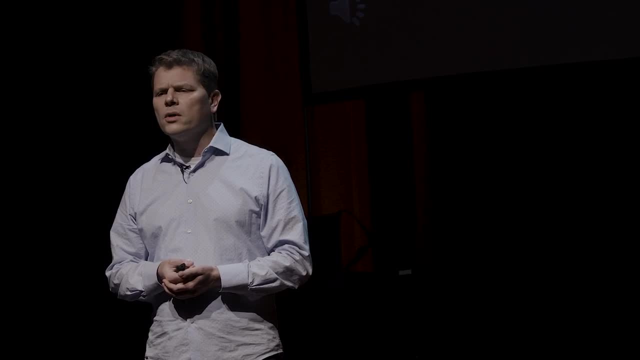 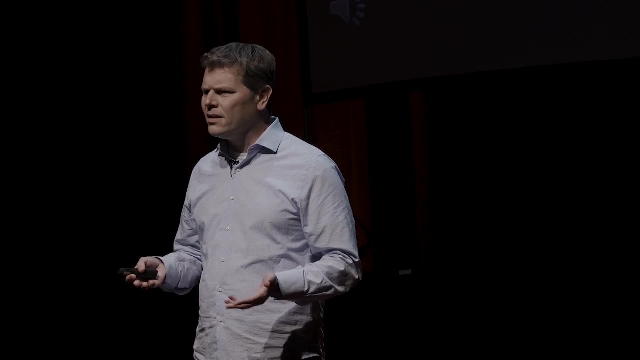 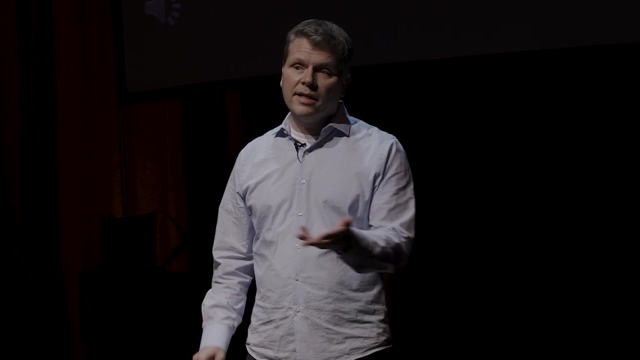 We see the biological connections in our newborns, who can recognize a musical beat at two or three days old and sense a missing downbeat in a rhythm pattern. We also know that our newborns prefer singing over speech and as adults we instinctively know this. 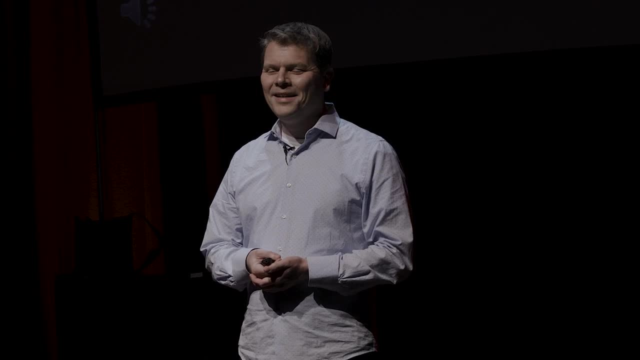 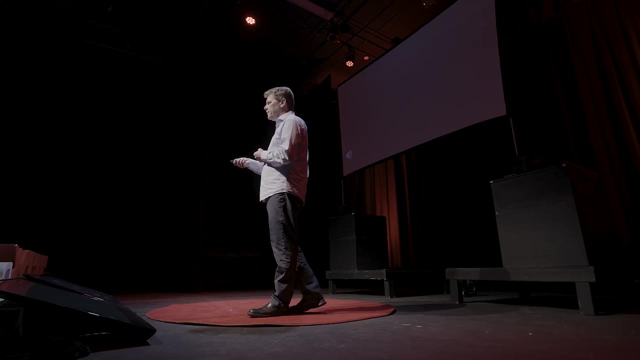 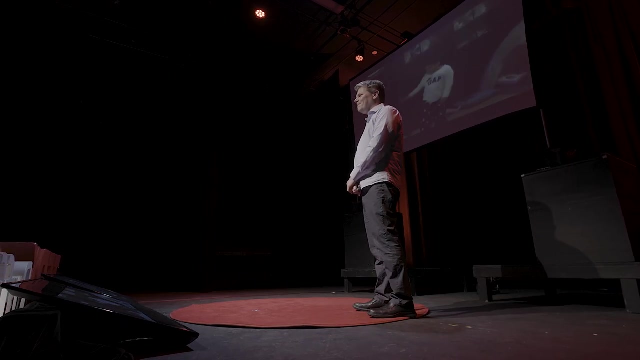 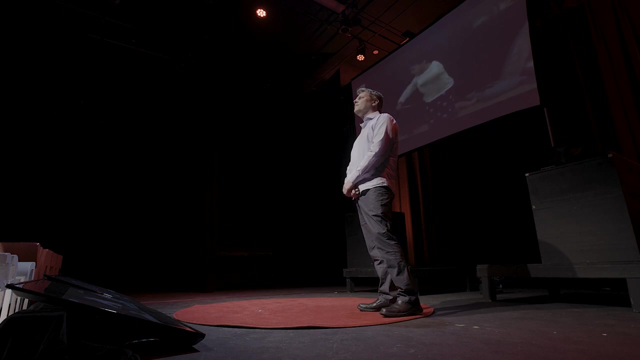 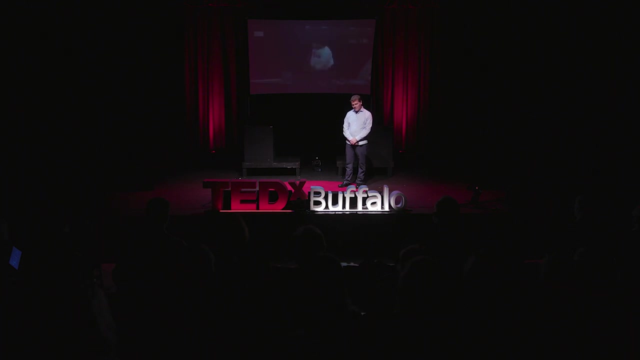 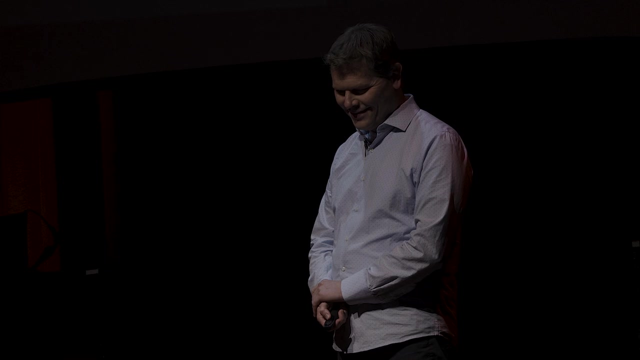 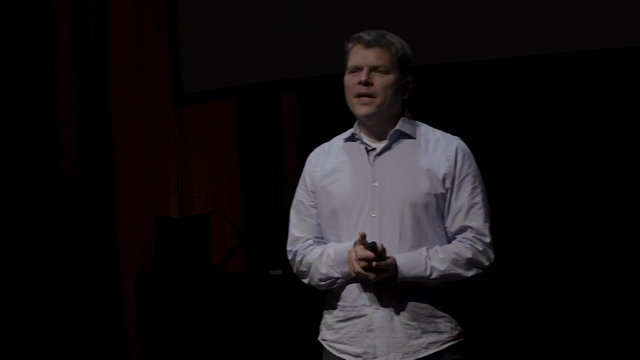 Which is why we launch into sing-song and sing lullabies to build emotional bonds with our infants and toddlers And reenact such a dynamic experience through a�. I love that ending. I've grown as a music educator That shared human response to music, so beautifully demonstrated in that video. 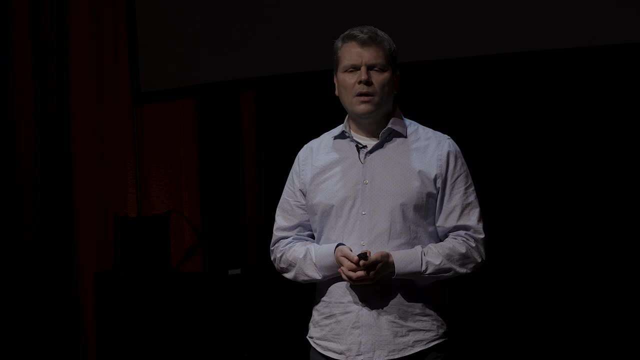 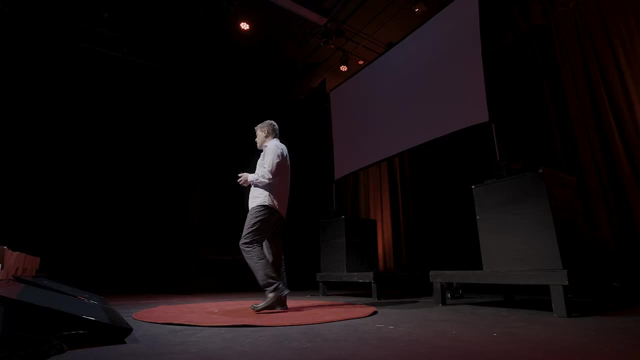 has become the driving force of music, force for my work. All of our kids can respond to and grow through the study of music and if, as the studies suggest, there's a biological and hardwired presence of music in us all, then our schools and communities need to be. 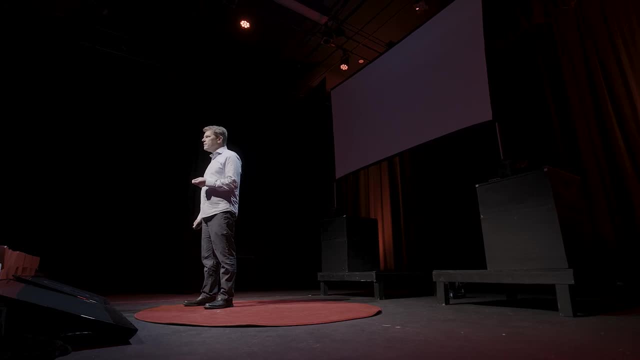 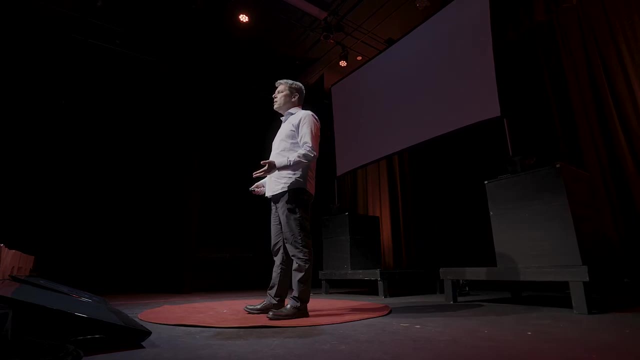 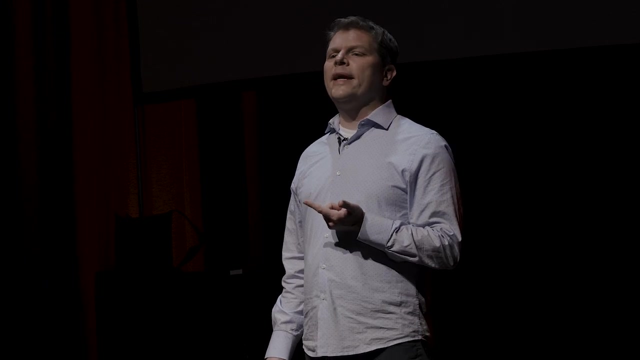 intentional in supporting that journey of discovery Beyond the biology. music advocacy is long centered on how the study of music contributes to success in other areas. Our music students learn to problem-solve, think creatively. Our students achieve higher grades in high school and on standardized tests. Music 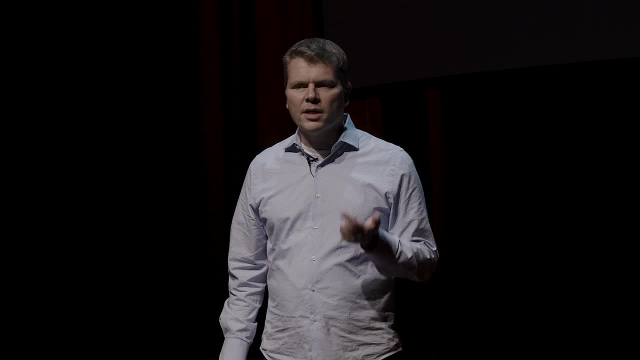 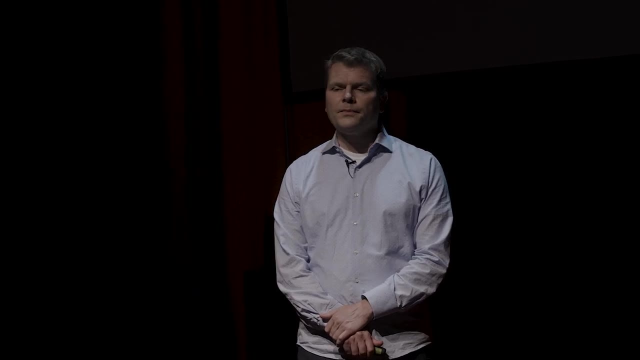 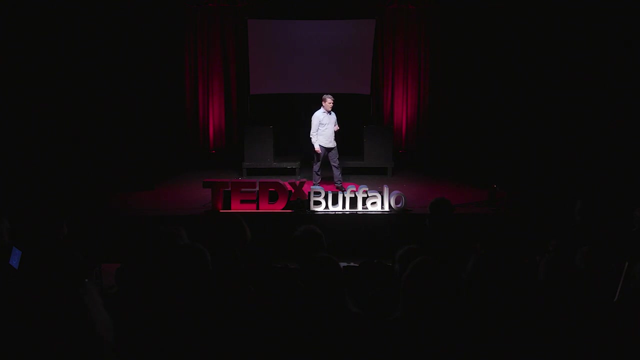 performance requires sustained effort, teamwork, discipline and encourages risk-taking—all skills valued by employers. But for me, the most important reason that music and music education should be a part of each and any type of work is that it is the most important tool for our students to be able to achieve their goals. 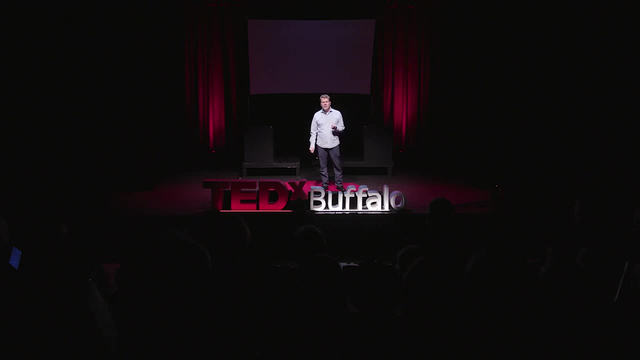 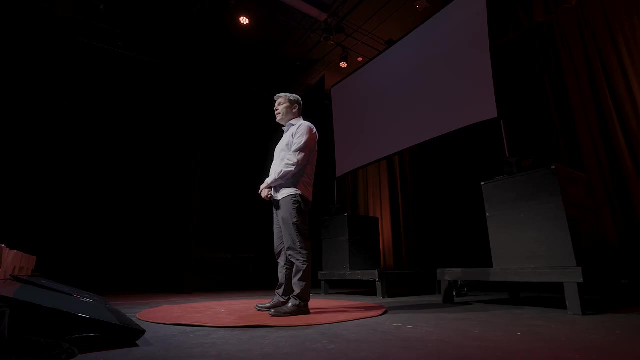 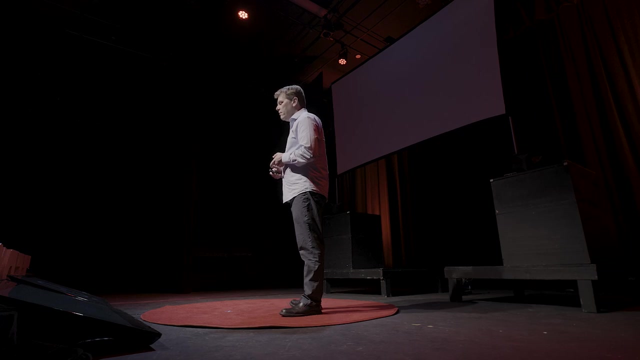 in every one of our kids' lives, especially in this changing world, is that through the study of music, our students catch a glimpse of other cultures And through that process they learn compassion and empathy for others. Music educators have long trumpeted these many benefits. 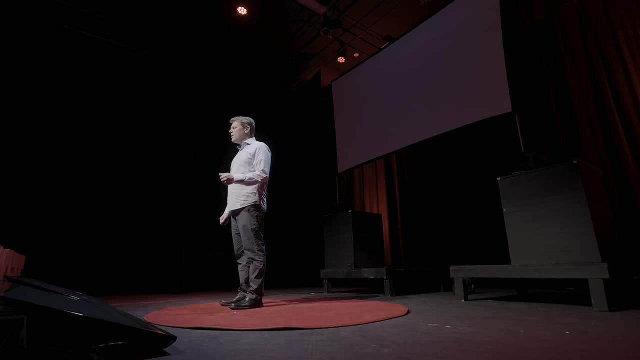 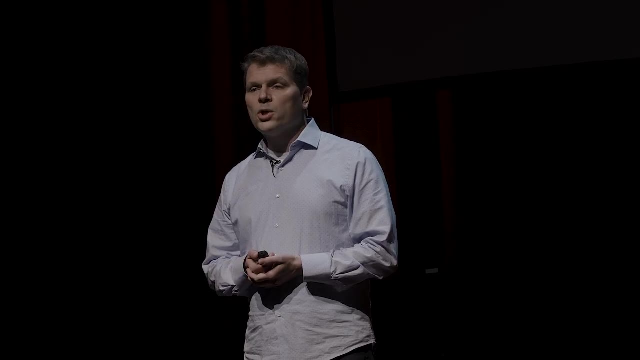 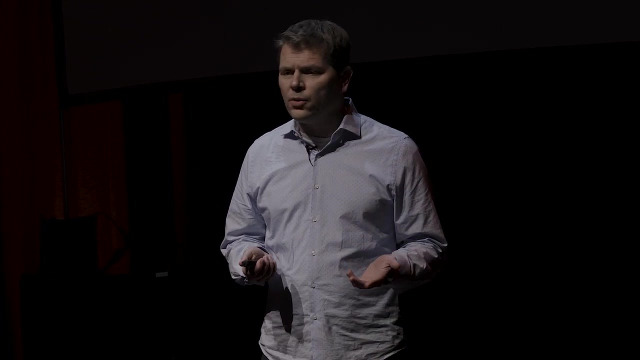 and yet, despite our efforts, there remains a troubling and frustrating disconnect between the research and school policy. Unfortunately, too many of our schools, and the culture of those schools, places music as an afterthought in the school curriculum and schedule, and too many of our musically inclined students. 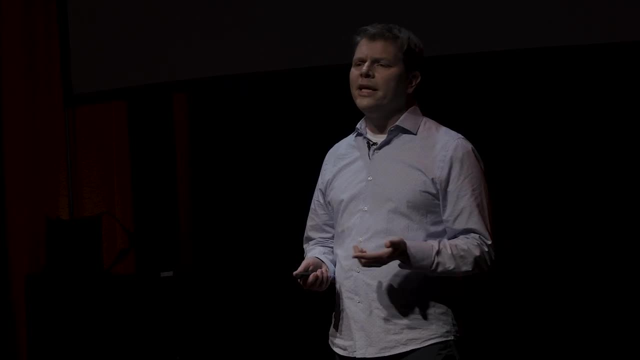 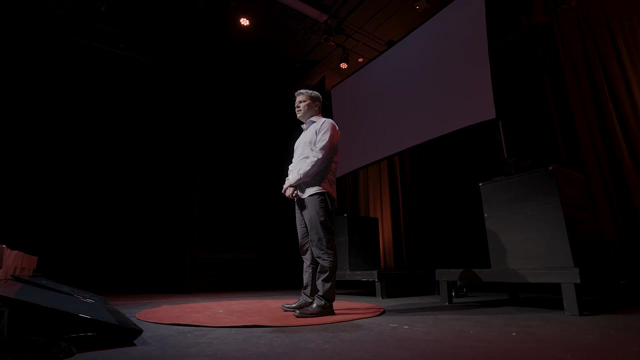 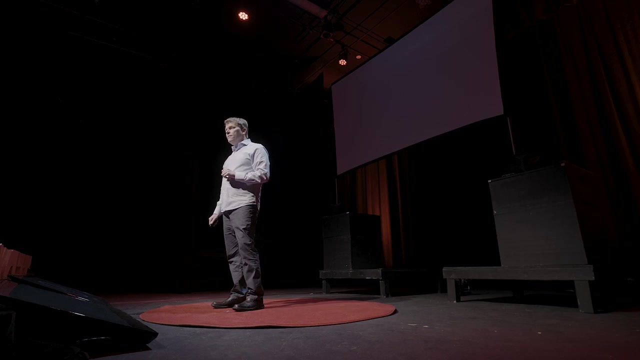 are made to feel less valued, when that musical inclination is simply a natural part of who they are. So what's the reason for this disconnect? I would argue that schools are primarily focused on adult priorities. Now, of course, schools are a reflection of the community at large. 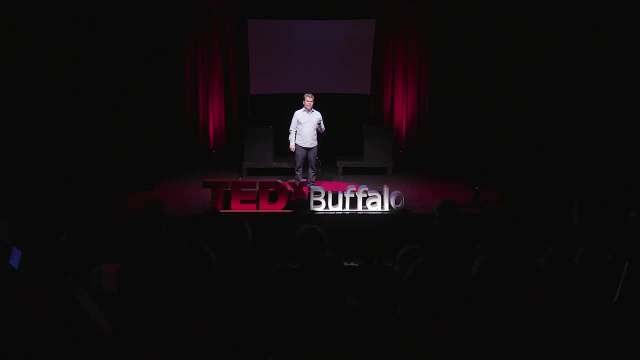 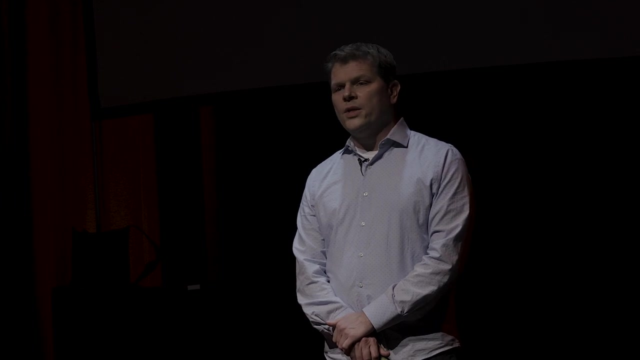 but I believe that our investments, the priorities, the culture of our schools need to be focused on the needs of the students first, not the adult wants and needs of the community. Now, I'm sure that our school leaders would certainly agree with that statement in principle. 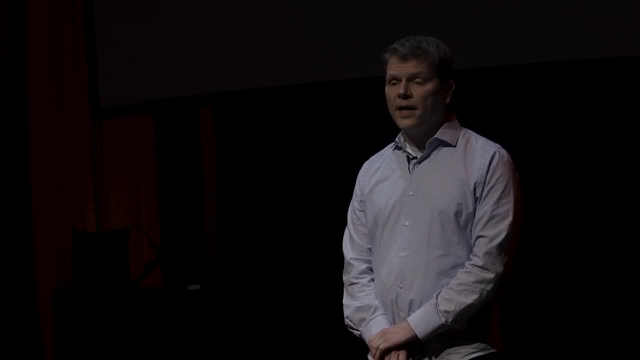 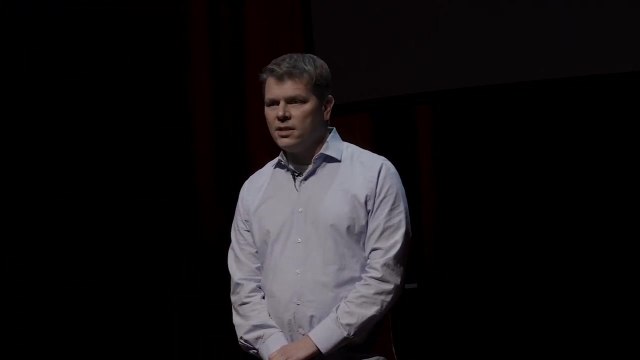 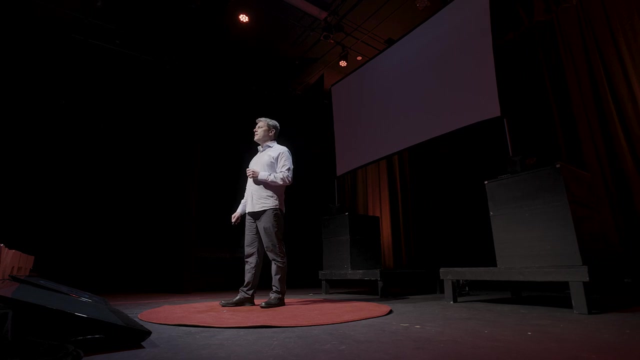 but in practice many of our schools fail to serve and support the needs of all students equally. According to the National Center for Education Statistics, only 29 states define music or the arts as a core academic subject. Six states have no arts requirements at all. 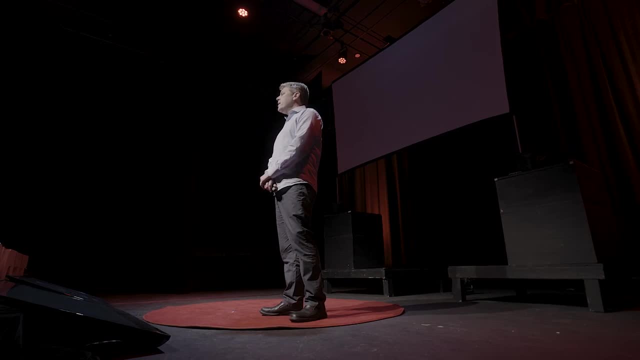 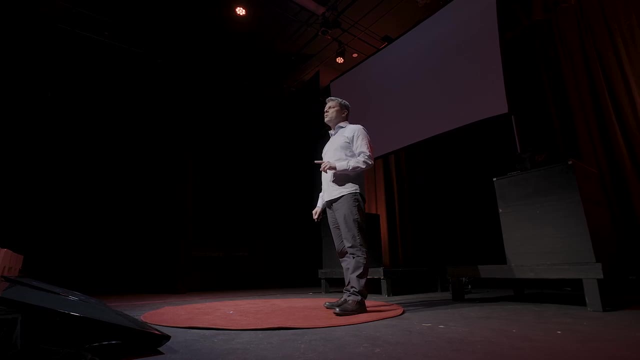 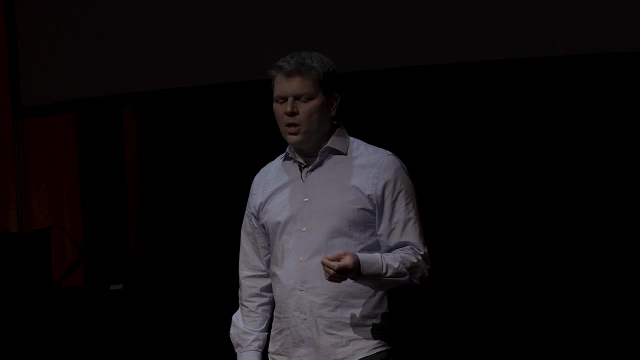 as part of their K-12 standards, And according to an analysis of the US Department of Education study in 2012,, there were 2.1 million students in a school that offered no music education. Now we know that schools are charged. 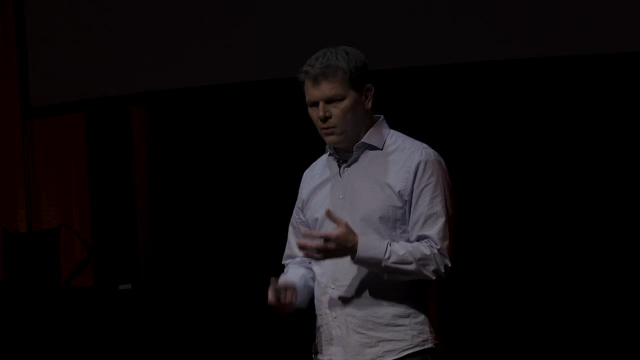 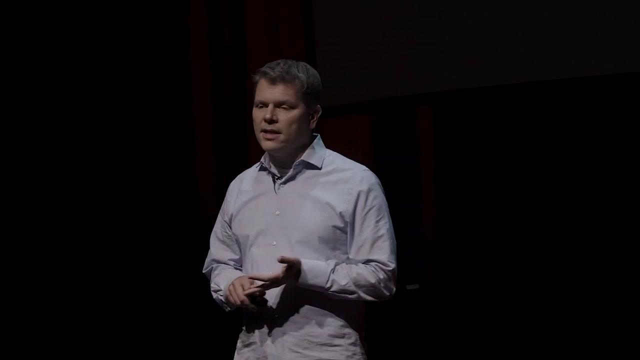 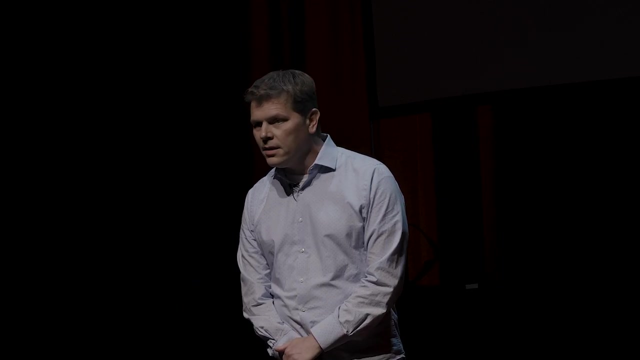 with meeting the needs of important mandated subjects that form the core of the school day, Subjects like English, math, science, which have an attached state assessment. More recently, STEM education has become a priority and our administrators need to respond to the pressures of those mandates as well. 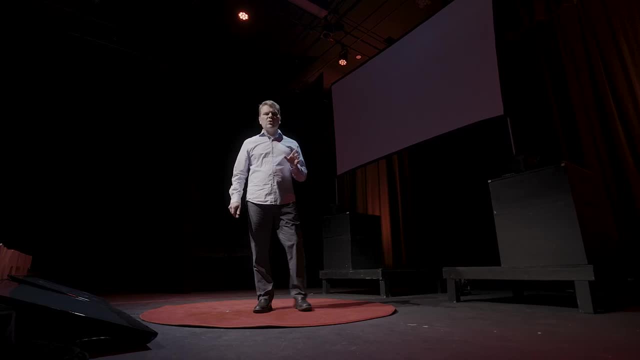 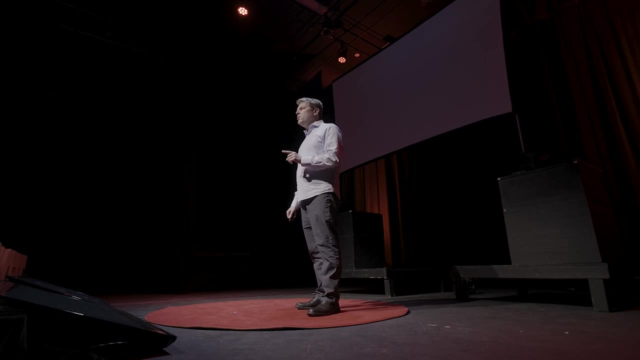 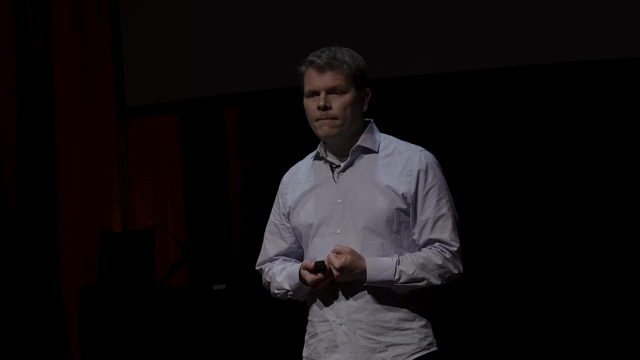 But beyond those requirements, our schools are also charged with making important curricular decisions about the remainder of the school day, And those decisions, those important local decisions, are deeply impactful to the lives of our students. I would argue that those remaining priorities are too much a reflection of the adults in charge. 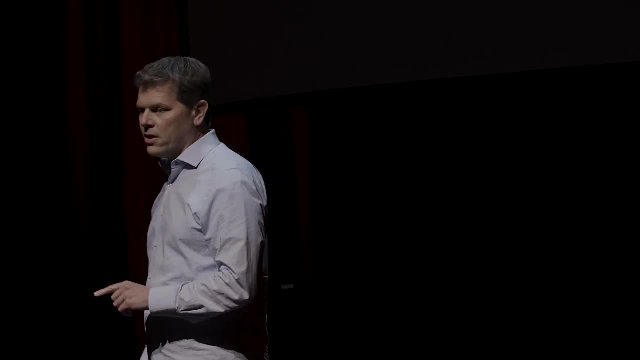 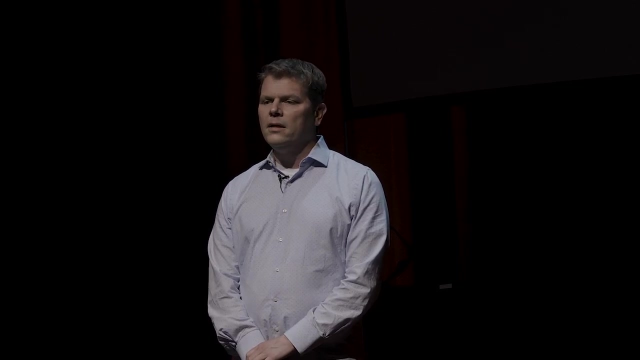 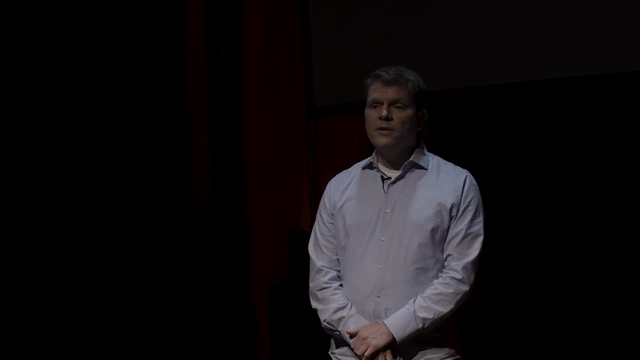 rather than the needs of the students in their charge. Programs like athletics, historically highly valued by adults and society, are given preference in the budgeting process, while music and the arts, less valued by adults, are frequently forced to compete for what's left. 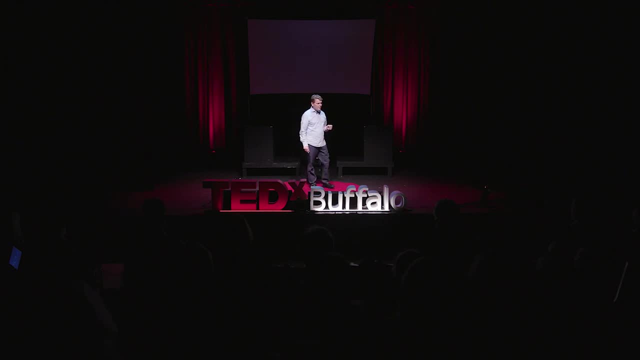 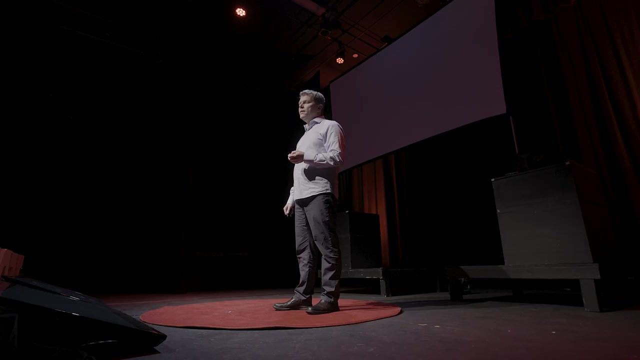 What's emerged, then in many schools is a budgeting process which is centered around protecting adult priorities while at the same time, solving financial issues on the backs of other, less popular programs, and all at the expense of student equity. Now, this isn't to say that there hasn't been 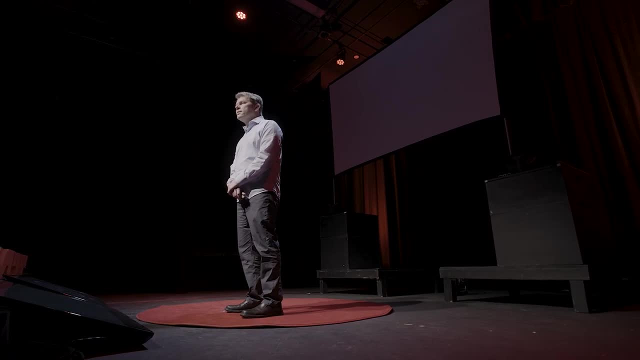 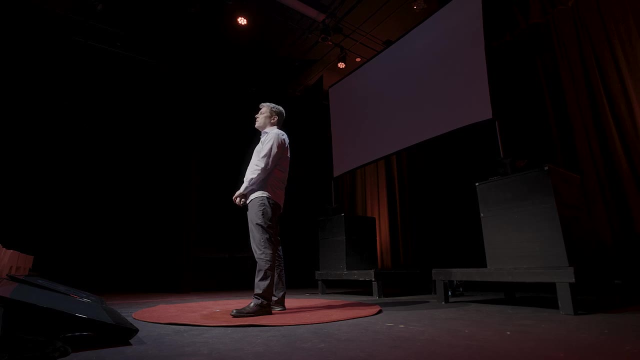 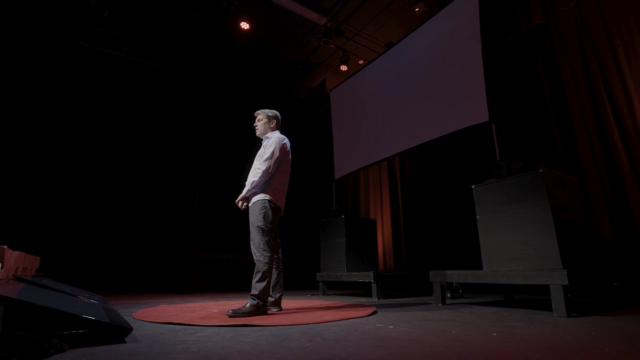 any investment in music or the arts There has simply that the investments made have frequently been out of balance and are easily at risk when a crisis occurs. Schools exist to serve the public and educate their children- all children. as a parent, Shouldn't you expect that your musically inclined child? 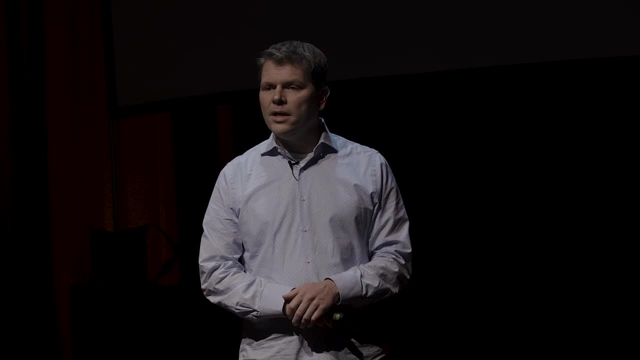 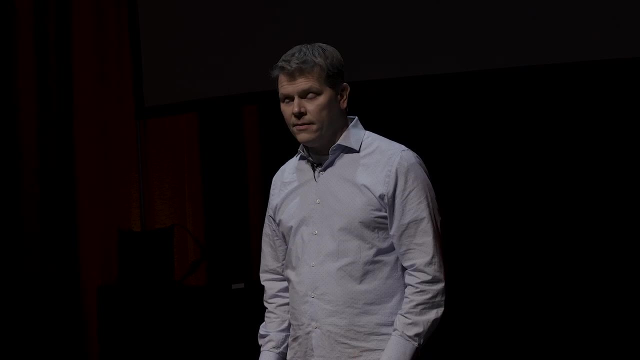 be made to feel just as validated and supported as your young aspiring athlete. If we are truly to see all students equally, then we need to look through their eyes. We need to budget, invest, prioritize, with each and every one of them in the forefront of our thinking. 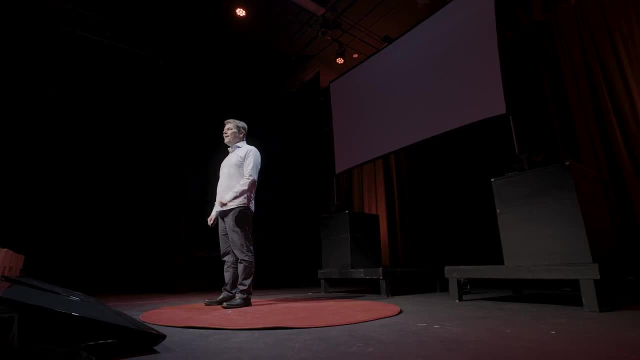 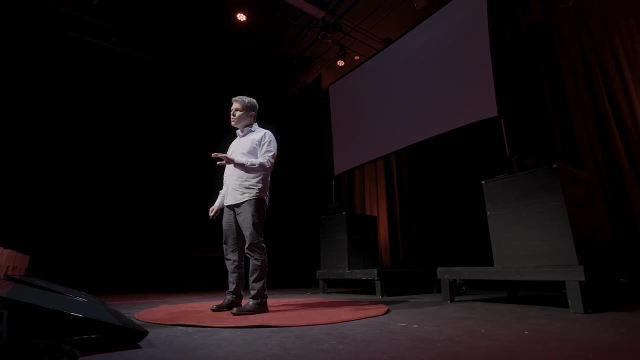 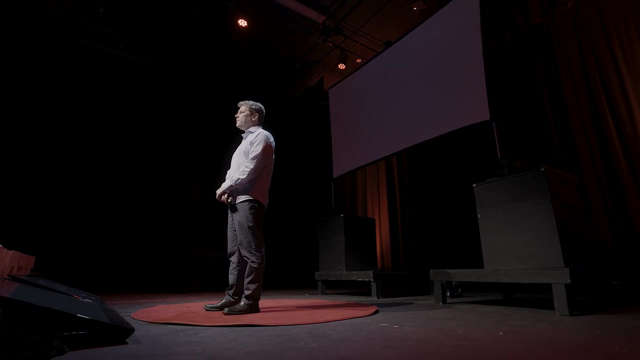 and we need to remove from that process any of our adult preferences and biases. We need our schools to be neutral facilitators, neutral in creating an environment of encouragement and acceptance for every student. The imbalance that we see in our schools as music educators, 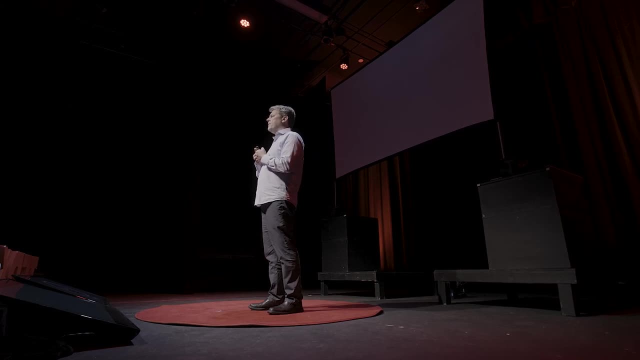 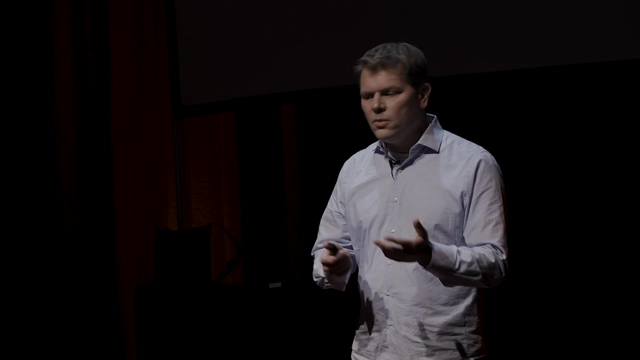 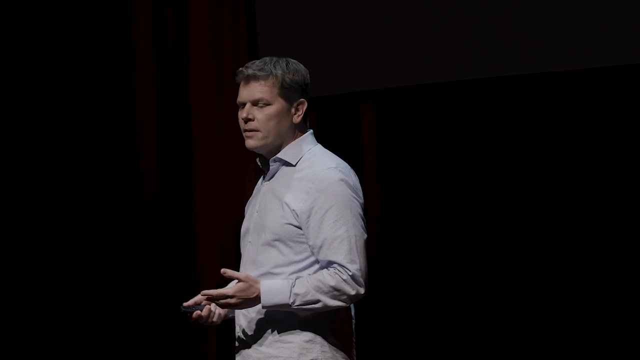 it affects us but more importantly, it affects our kids. It affects our kids and their sense of self. Our kids respond to what they see and what they hear around them. They respond to the adult priorities that are around them in their school. 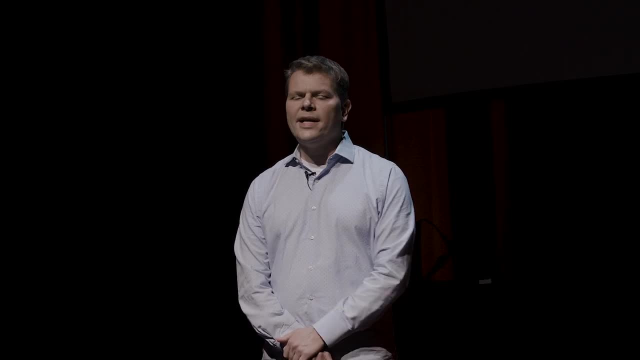 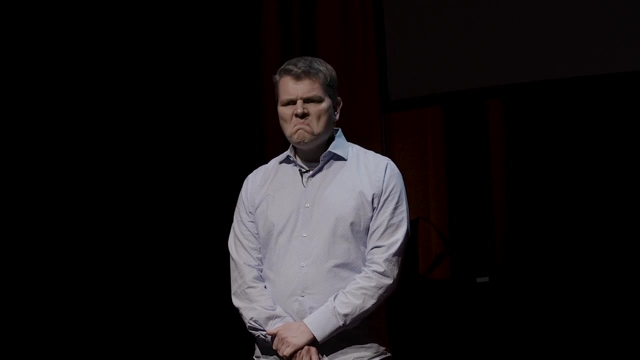 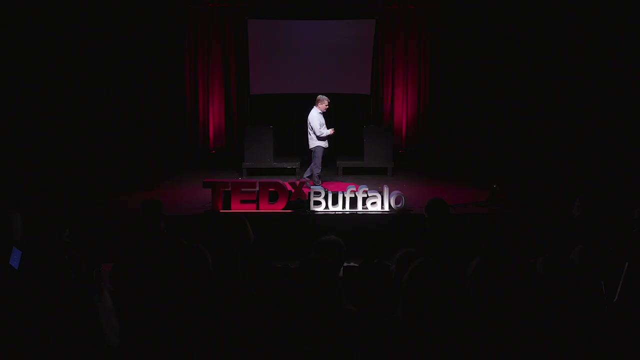 How are they made to feel if their natural curiosity, passion for music or the arts isn't reflected around them? How are they made to feel when they walk through the hallways and they know that they aren't a priority? I would suggest to you that. 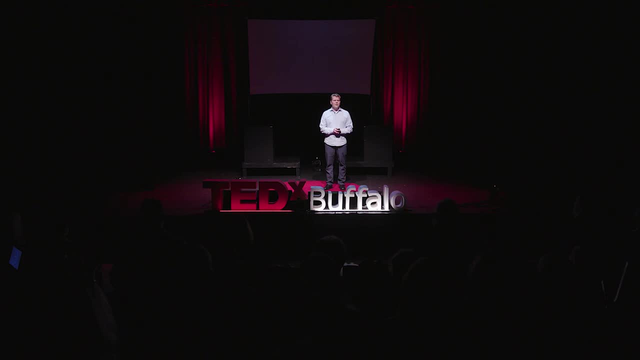 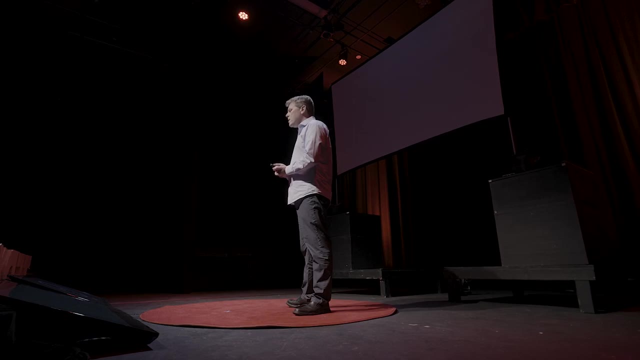 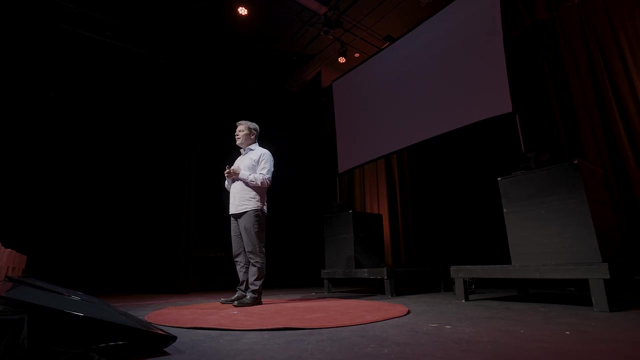 what we need to do is work on our kids' mental health. in that regard, A few years ago a TV personality did a story about young Prince George and how he loved, he loved- to take ballet as part of his school curriculum. She then proceeded to laugh. 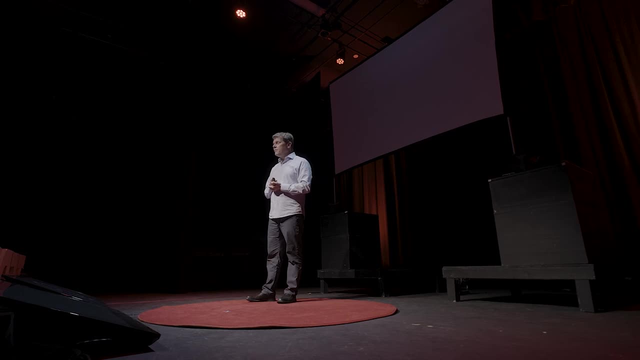 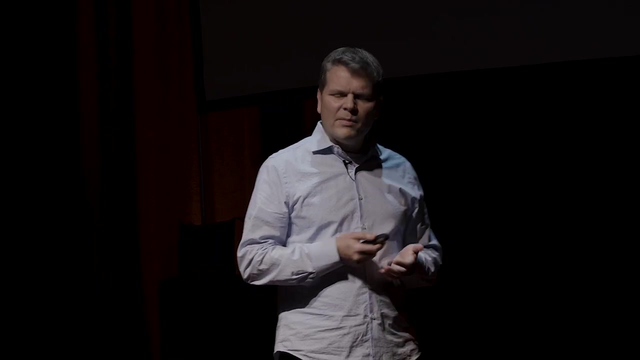 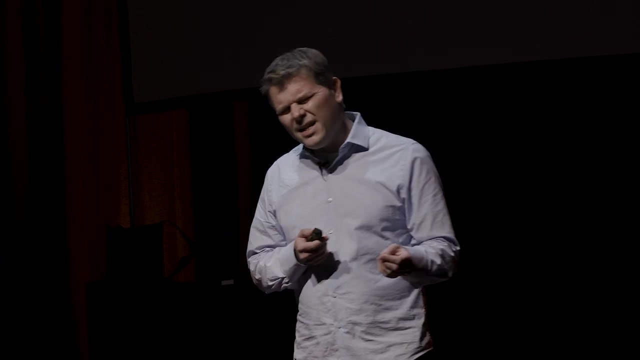 asking how long that would last mocking a boy for enjoying dance. Now, on the surface, that statement seems harmless enough, but in truth it's indicative of the kinds of cultural hurdles that we, as adults, can place in front of our kids who choose the arts. 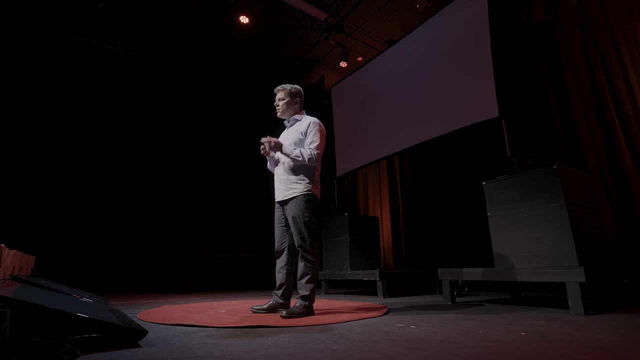 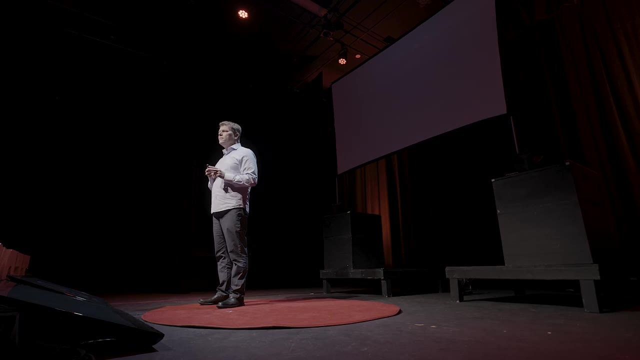 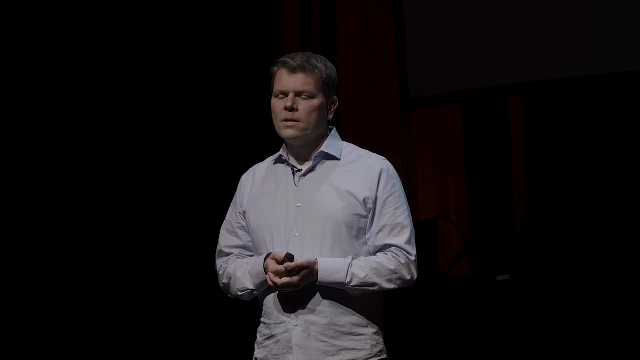 In both implicit and explicit ways. those kinds of statements and judgments are made by adults every day in schools and communities around the world, And again, all at the expense of our kids' mental health. We must do better. We all yearn to belong. 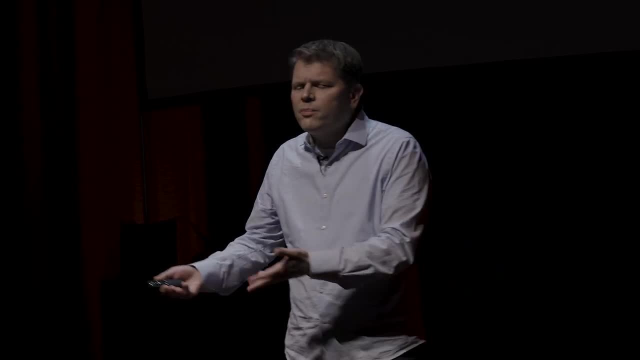 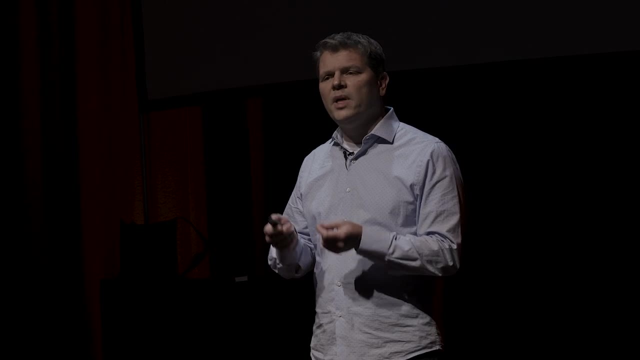 As music educators, we want our kids to walk the halls proudly, knowing that they belong. We're asking for the resources to support our work. We're asking that music be an equal part of the school day. We're asking for acknowledgement and respect. 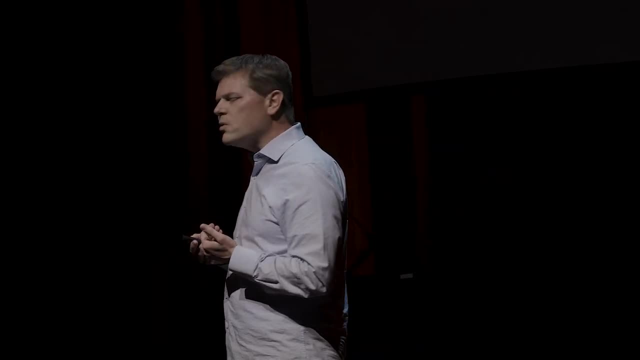 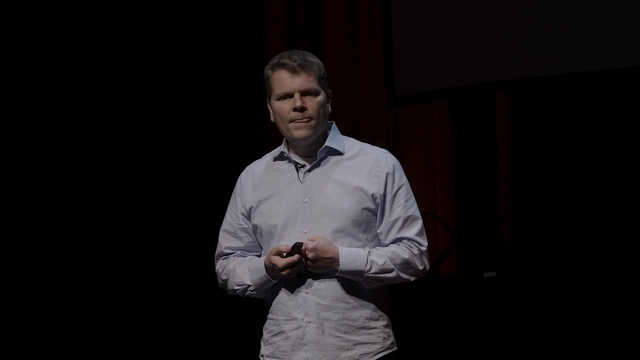 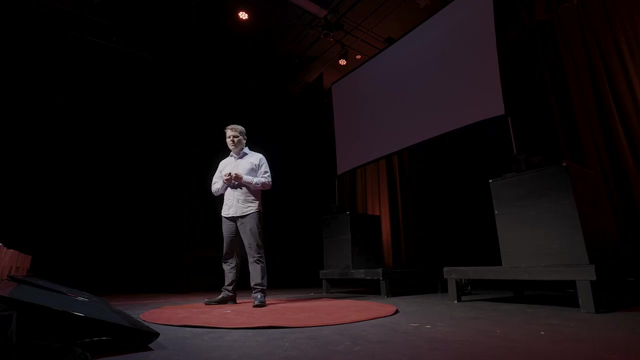 but we don't ask those things for ourselves as teachers. We ask those things for our kids, on their behalf, so that they can feel the same sense, same sense of pride and belonging as their peers. What we need to do is we need to look. 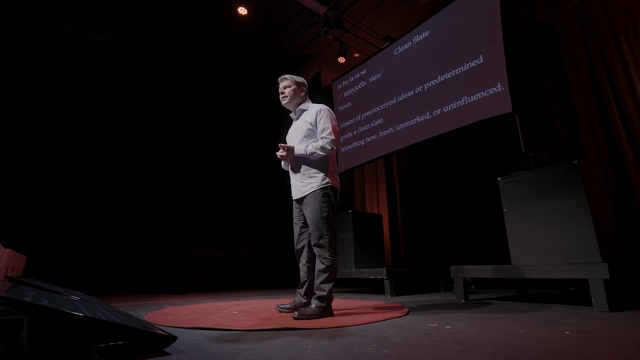 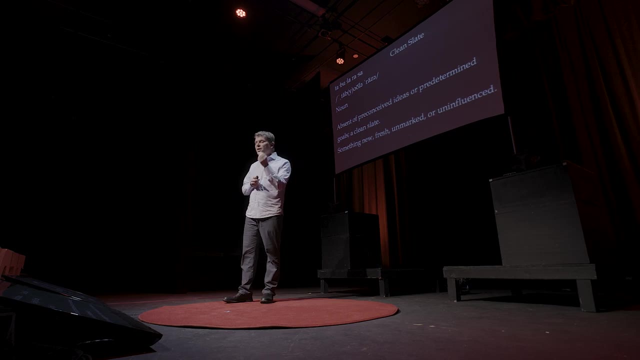 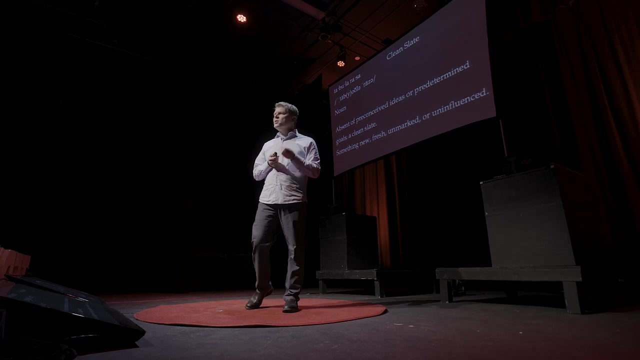 at each of our kids as a clean slate, absent of preconceived ideas or predetermined goals, something new, fresh, unmarked or uninfluenced. This is the change that we need. This is the change that we need: The statement that 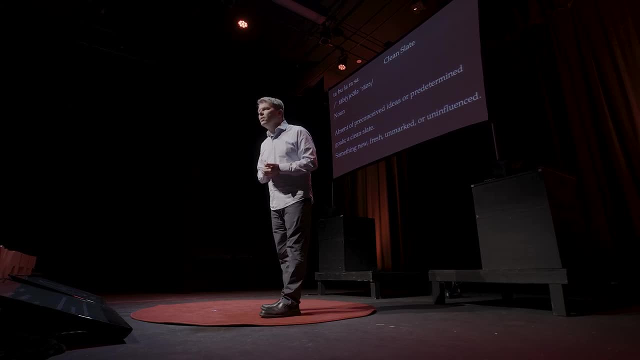 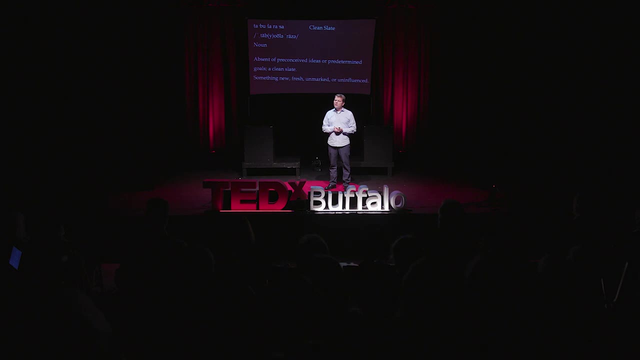 well, we've always done it. this way is no longer acceptable, when that status quo has meant no or inadequate music education for millions of children. What if we did this? What if we looked at them as something new, fresh, unmarked. 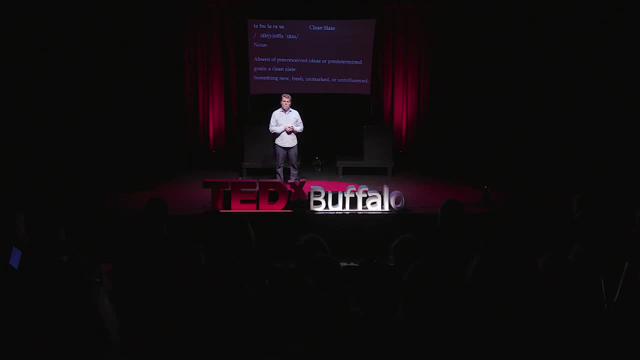 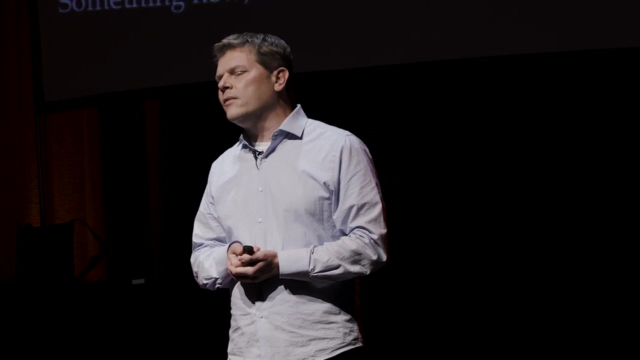 or uninfluenced. What would our schools look like then, with that change in mindset? If we did that, schools would make decisions which would validate our kids' natural curiosities and give them permission to embrace their authentic selves. With that change, 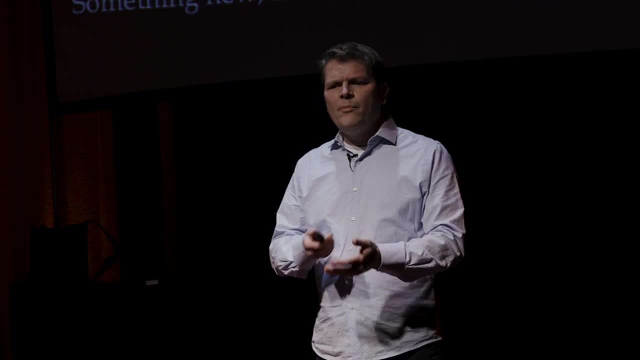 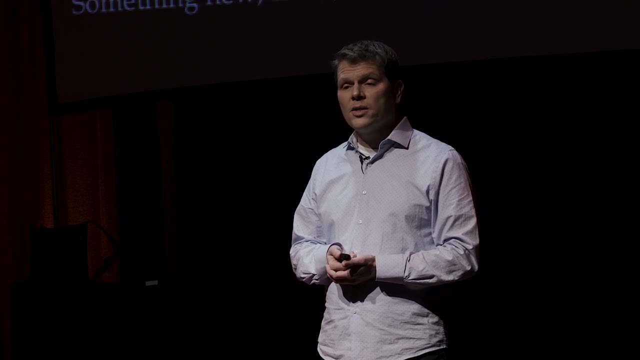 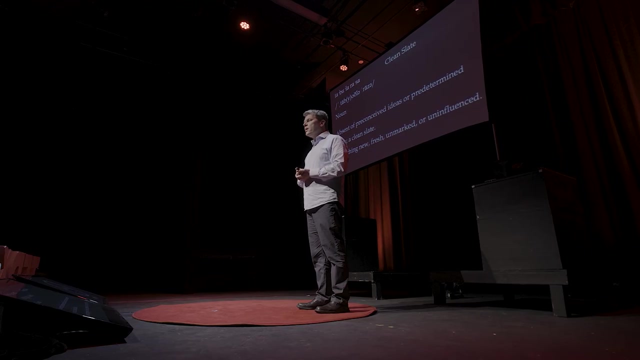 our kids and our schools would have policies which would validate every student choice. With that change, we would truly make room for music in the arts while uplifting all of our kids. Music can transform lives. I see it every day with my kids.